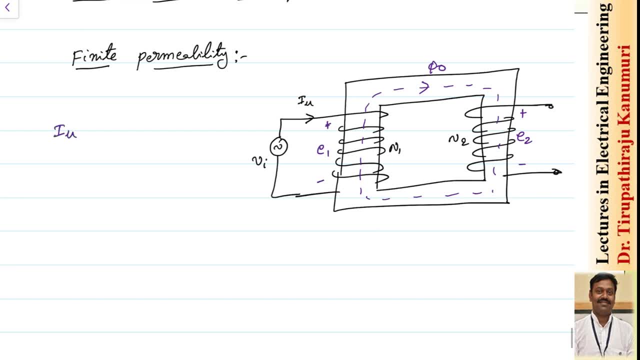 let us represent this current or the magnetizing component of current, that is, I mu, which is the magnetizing component of current, or this is responsible for the production of magnetic flux. Again, I am assuming that the amount of copper losses or the resistance of the conductor material 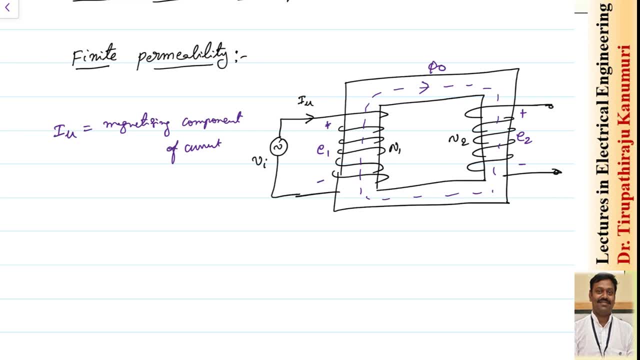 or it is a pure inductor and there are no any other type of losses. Only permeability is finite. there is no other losses in the system or in the transformer. So let us represent this value of this magnetizing component as I maximum sine omega t. So let us take it as the reference wave. 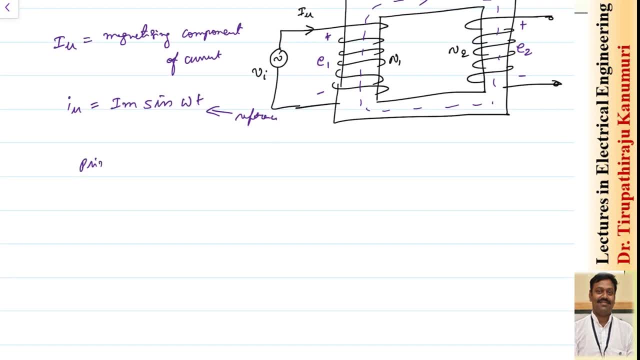 So reference wave. So now, because of this, the mmf will be produced in the primary that is given by primary magneto-motive force. This will be equal to number of turns in the primary is n1 multiplied by the magnetizing component of current. So this will become n1 into. 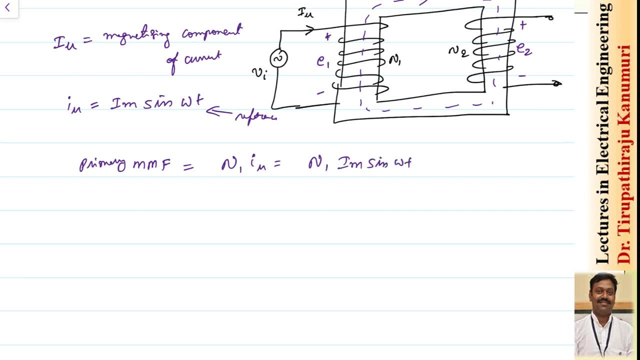 I maximum sine omega t. So from this I can calculate my primary flux, or this is also called as main field flux, because multiple fluxes will be there. One flux will be due to secondary and primary component to compensate for the load. We are going to see all those things in coming sections. 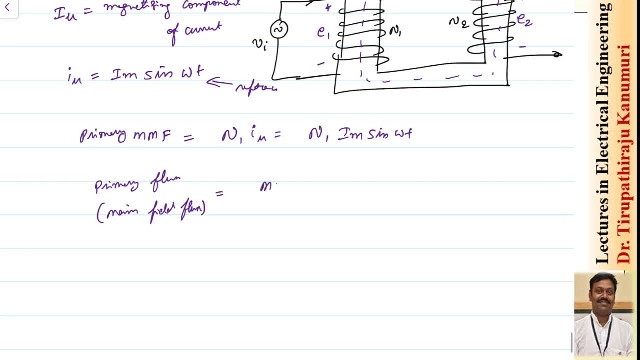 today's lecture only. So this primary flux that will be produced will be mmf divided by reluctance of your material, because reluctance is finite. So that is why this will be equal to n1 I maximum sine omega t divided by the reluctance. So this n? I maximum by 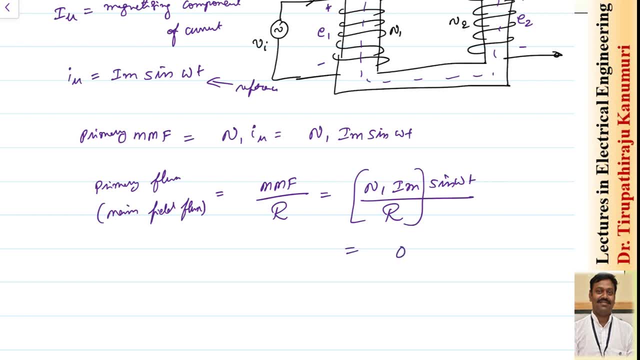 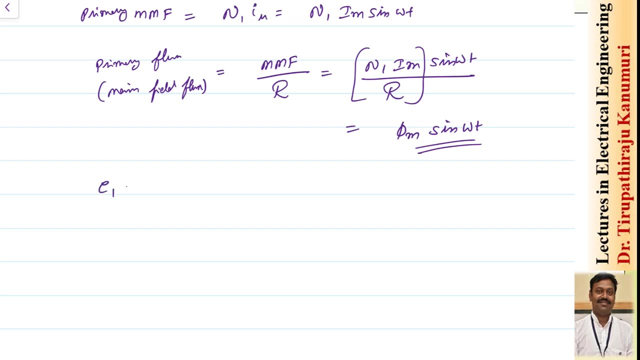 r. I can represent by because I maximum is there, so I can represent it is phi maximum, phi maximum sine omega t. You can see here the flux is in phase with the current phase r. Whatever is the current phase r, the flux will be in phase with this one. So now the emf induced in the primary. 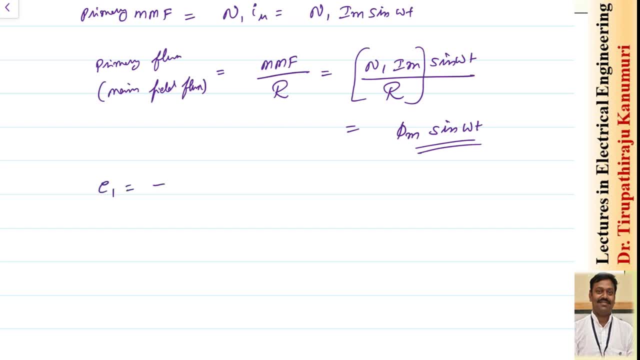 flux will be as per Faraday's laws of electromagnetic induction. it will be proportional to rate of change of flux. linkages, or e1, will be minus of number of turns in primaries m1 into d5. by dt or this I will become equal to n1 into rate that phi we have to differentiate with respect to. 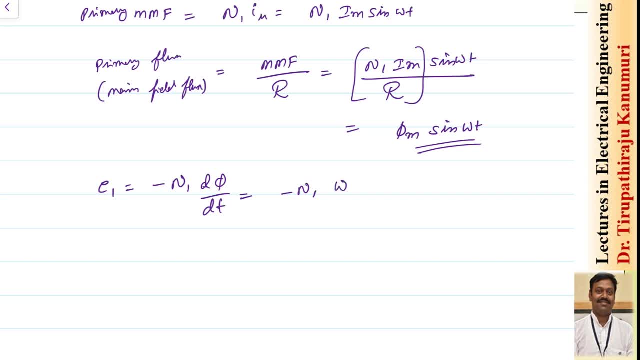 time. So when you are differentiating this with respect to time, you will get it as omega into phi maximum, into cos omega t or this I can write as minus sign I can take inside. So this will become omega into phi maximum sine of omega t minus 90.. Actually, cos omega t I can write as sine 90 minus. 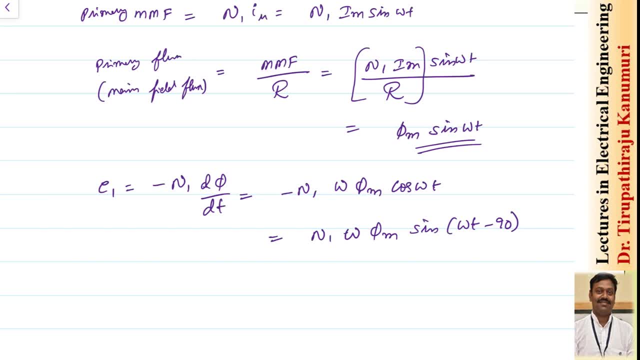 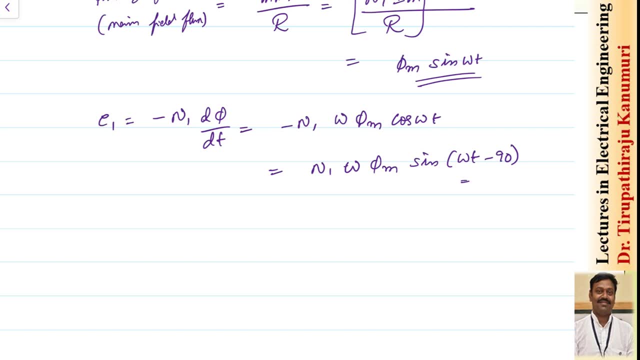 omega t, that minus I am taking inside. so inside angle becomes opposite Getting it. So that is the reason I have taken inside, So that I can compare this with the flux wave. What is the relationship between the flux wave and the emf wave? So here you can observe that emf phase r. 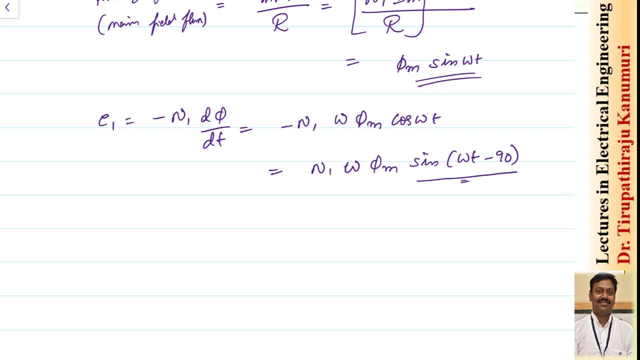 is lagging behind your flux phase r by 90 degrees because minus 90 is coming here. You agree with me. So this you have can expand this one. This omega is nothing but equal to 2 pi f, So this will become equal to 2 pi f into n1, into phi maximum, into sine of omega t minus 90 degrees. 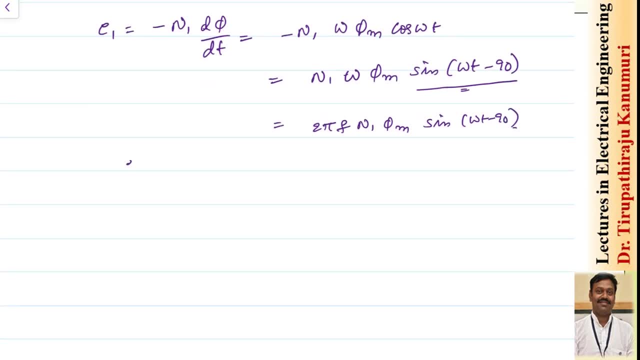 So similar way emf will be induced in the secondary also. So emf induced in the secondary will be minus n2 into d5 by dt. So equation: if you substitute you will get it as 2 pi f into n2, into phi maximum, into sine of omega t minus. 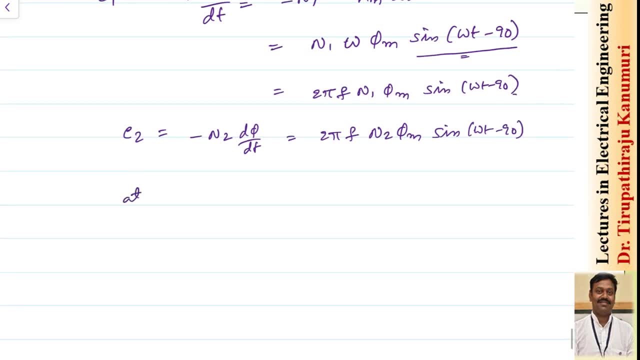 is 90 degrees. everyone agree with me. so now, at omega t is equal to pi, the value of e1 will be equal to n1 into phi maximum, into omega. omega is nothing but 2 pi f into sine of now, omega t is equal to pi. so this will become pi minus pi by 2, because 90 is nothing but pi by 2, so pi minus pi. 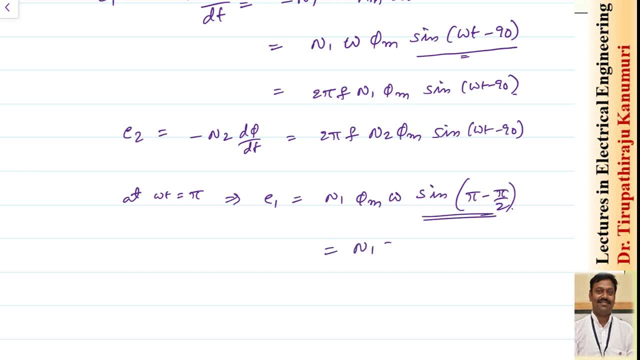 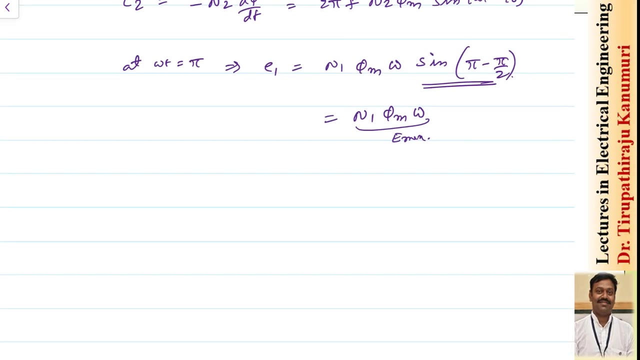 by 2 is sine 90. sine 90 is equal to 1. so this will become n1, phi, maximum omega, or we can tell it correspond to maximum value of the emf. so this i am representing by the term as e maximum value. so practically all the values are represented in rms values. so the rms value of the emf induced. 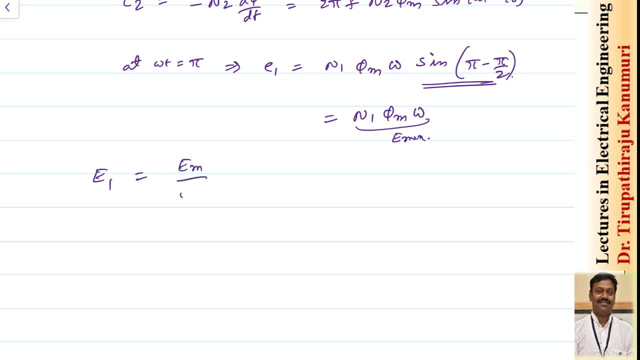 will be maximum value or e maximum value divided by root 2. so this will become equal to root 2 times of pi f, n1 into phi maximum. so root 2 pi will become 4.44 f into n1 into phi maximum. ok, Similar way I can calculate my value of E2 is equal to E maximum 2 by root 2, this also will. 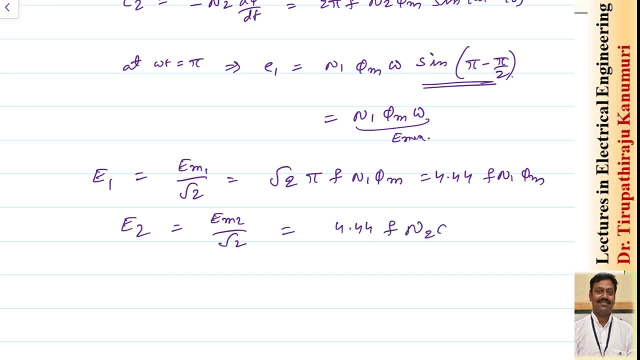 be equal to 4.44 F into N2, into phi maximum value. So now to calculate the flux, sometimes in the numerical, they will give the flux density and the area. So the flux can be calculated by the product of maximum flux density multiplied by the area of the core And while taking the area, 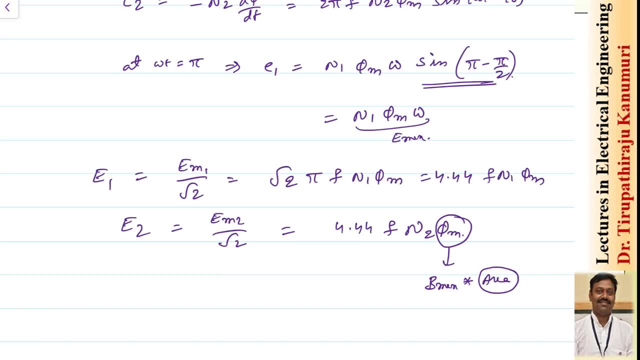 of the core, because I told you that the core is made up of laminated steel. in the lamination between two laminates we apply some insulating material. That insulating material will not be responsible for production of flux. So we have to take the net cross-sectional area. We have to 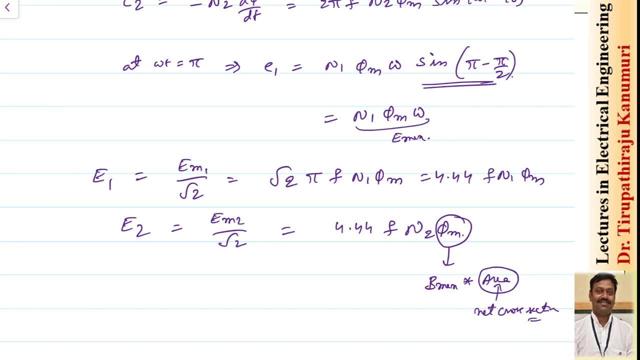 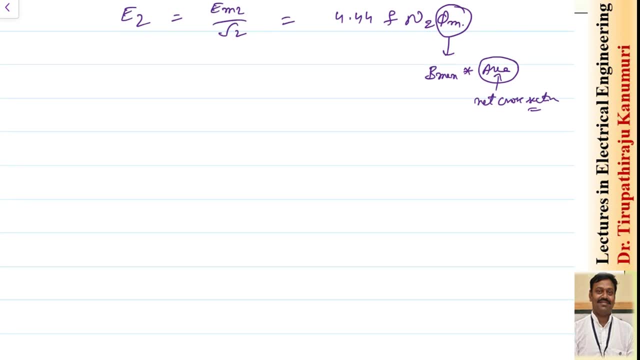 take the net cross-sectional area of the core, not the gross cross-sectional area, because only that is responsible for the passes of the flux. You have to remember this one. So now, if you are drawing the phasor diagram for this, if this is my flux, the flux will be in phase with the 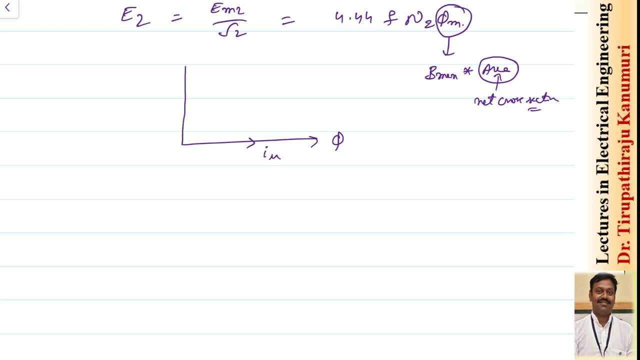 magnetizing component of current. So this magnetizing component of current will be lagging behind the flux. So if this is my flux, the flux will be in phase with the magnetizing component of current. What does this mean? This means that the flux will be in phase with the magnetizing 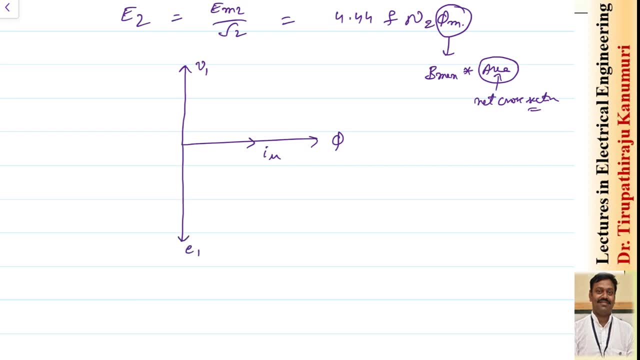 component of equal quality spectrometer where the flux is in phase with the magnetizing component of the magnetizing component. So this is the DC current度. So when the compact current is busy, the flux becomes low and the liquid relationships with the global spectrometer. 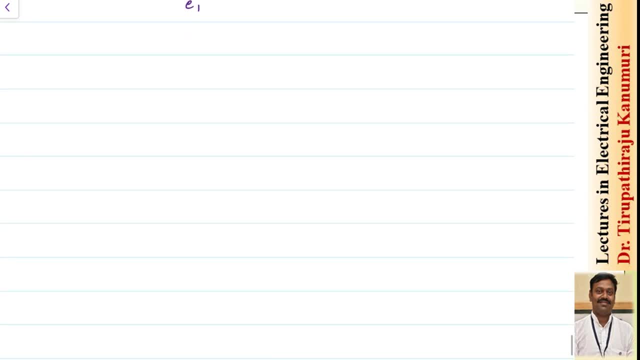 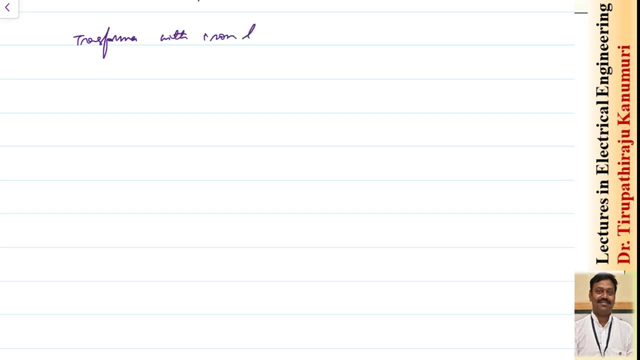 in one phase ruin this. So thus this is the external circuit. If we put cooking material mass into the master generation states for heating, then our result must be having ну 2 times mu回 steak output. Fr, C, the flux мире for heating광 yêu. 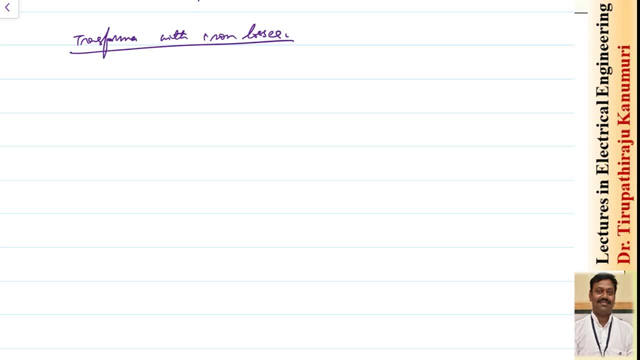 So the name is telling us the iron losses. This iron losses corresponds to the losses that happens in your core, because the transformer core, whatever core is there, this material is also a metal because when the flux is passing, that flux is linking with this core also. 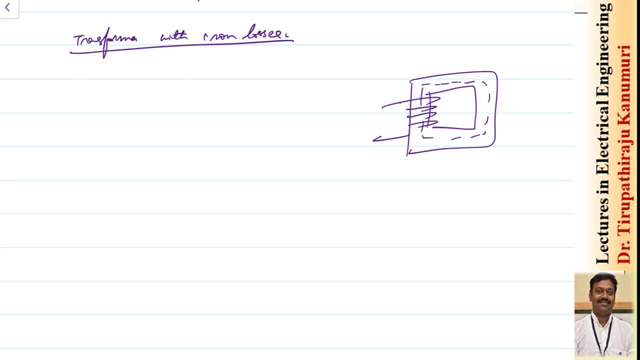 So because of this, the EMF will induce in the core also and that leads to the circulating currents, which are called as the eddy currents. They will be in the circular form or in the form of an eddy. That's why they are called as eddy current. 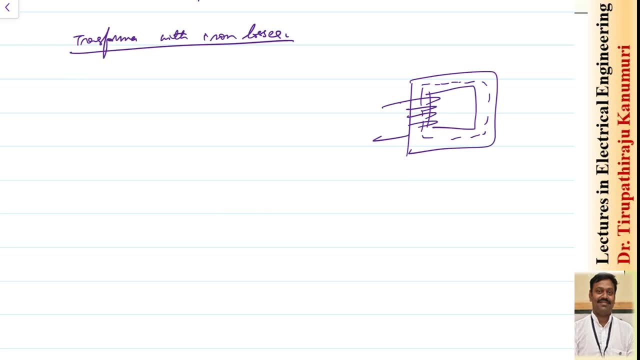 Because of that eddy current- again I square into resistance of the core material. for eddy current, some circulating currents, the heat will be produced. That loss is called as eddy current loss. The eddy current loss happens in the core of the material. 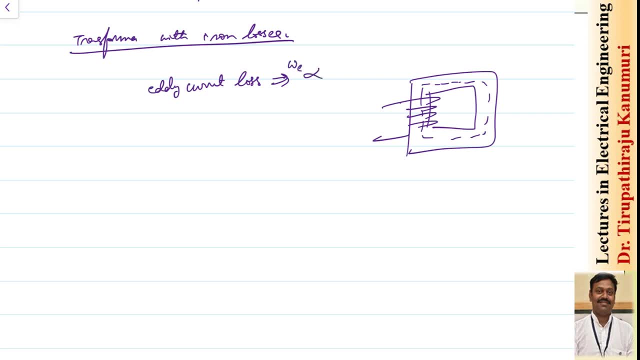 So this eddy current loss is proportional to this, is represented by WE. So this is B maximum square. F square into T square. So B maximum is the maximum flux density, F is the frequency and T is E Thickness of laminations. 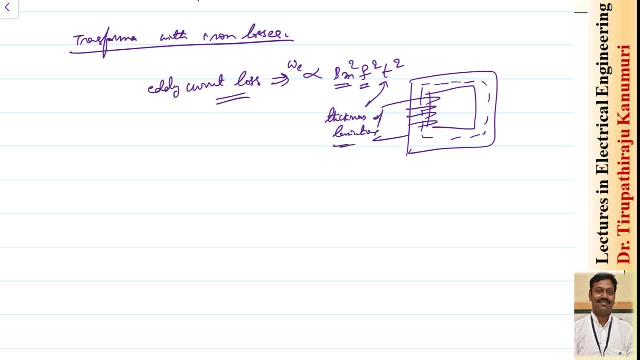 So if you want to decrease the eddy current loss, the thickness of lamination should be as minimum as possible and the flux density should be minimum and frequency should be minimum. Now coming to the second type of loss, because no material follows the normal linear characteristics, 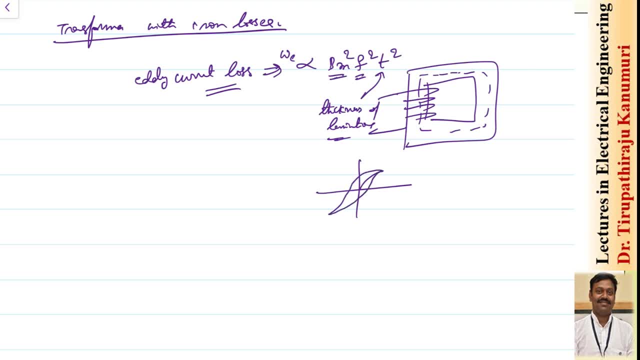 I have told you that there will be BH characteristic like this, or this curve is called as BH curve or hysteresis curve. This is the magnetizing component versus the flux curve, So it doesn't follow The linear curve. it forms some area. 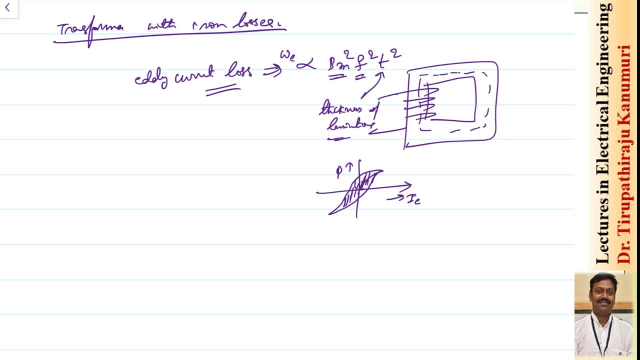 So this area under this curve gives what is a loss per each cycle per volume. What is a loss in one cycle per unit volume of your material? That means we are taking the sine wave. in one cycle, How much loss is coming? That is represented by the area per unit volume. 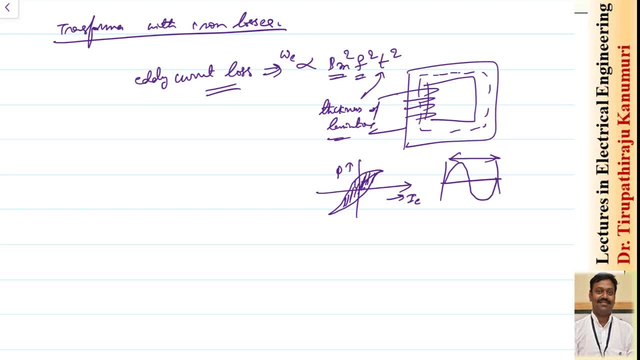 You have to multiply with the total volume, that gives how much is a loss per cycle. So this is called as hysteresis loss. So hysteresis loss is proportional to B maximum, to the cover of X into F, into V. F is the frequency, B maximum is the maximum flux density and V is the volume of core material. 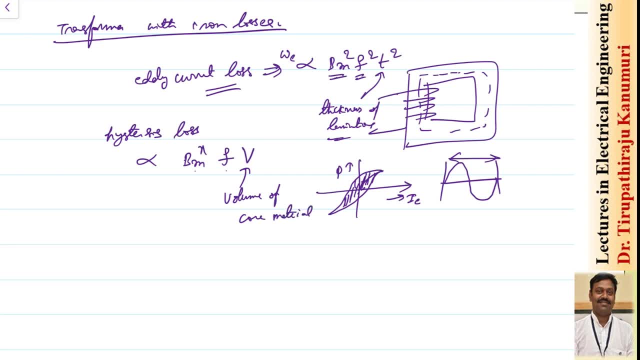 More the volume of the core material, more will be the hysteresis loss, And this X is a constant which depends on the type of the material. This is called as hysteresis constant, Generally for silicon, steel or electrical steel, this value of X will be equal to 1.6. 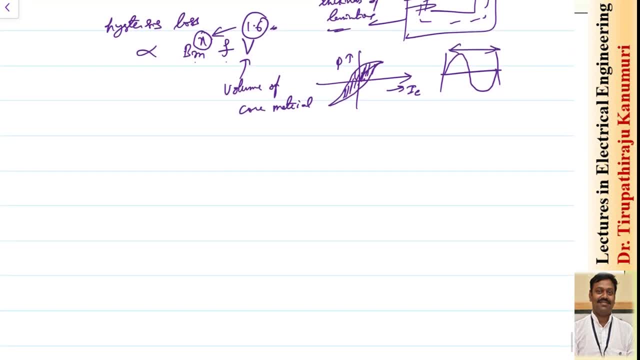 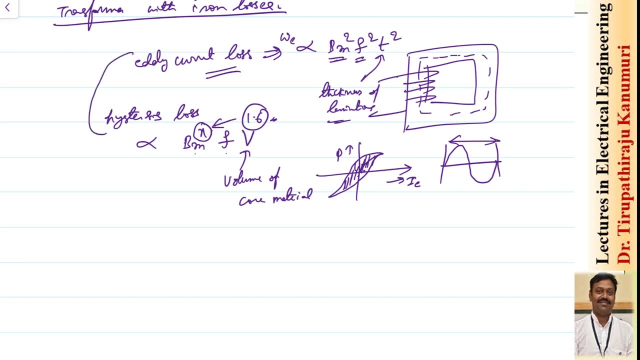 in practice. Okay, this is about these losses. Now, both these losses, whatever losses are there- they are produced in the core- That's why they are called as the core losses- or they are produced in the iron material. They are called as the iron losses. 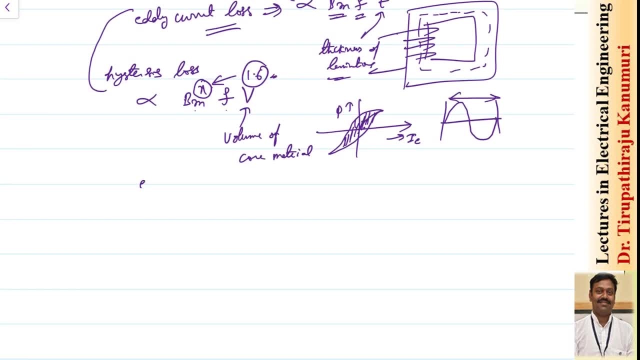 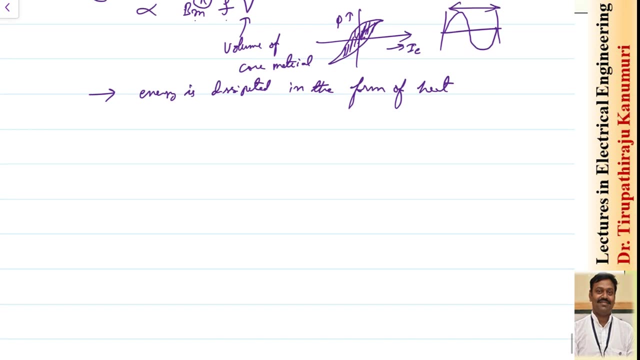 And both these losses. the heat is produced or we can tell that the energy is dissipated in the form of heat. That means they dissipate the active energy in the form of heat. So, if you remember, we have seen, in the case of electrical circuits or AC circuit analysis. 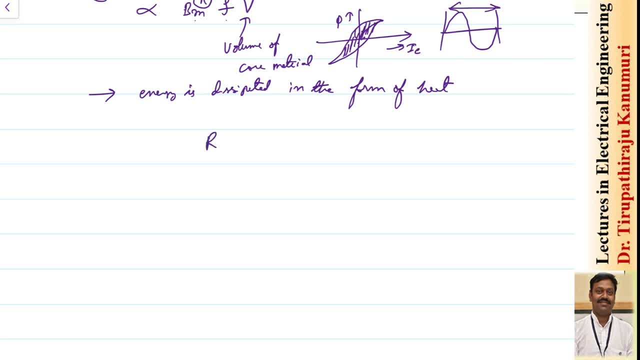 we have taken electrical engineering. there will be three items: One is the resistance, second one is inductance and the third one is the capacitance. And inductor and capacitor doesn't consume any power. They will take the power for one quarter cycle and return back for another quarter cycle. 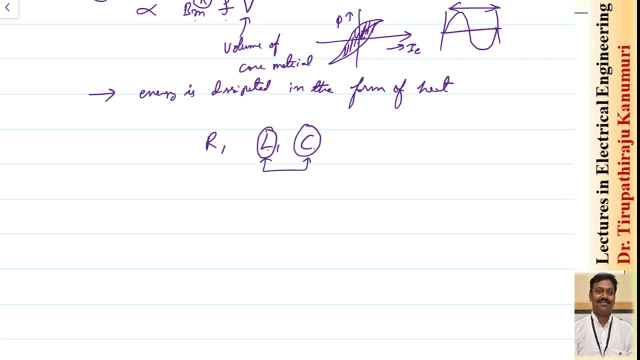 These things we have already discussed. What is the effect of inductor or the capacitor in the systems? You can please refer there And we have seen there. the resistance will dissipate the power in the form of heat or heat. The resistance is responsible for the active power loss, or they can be represented in the 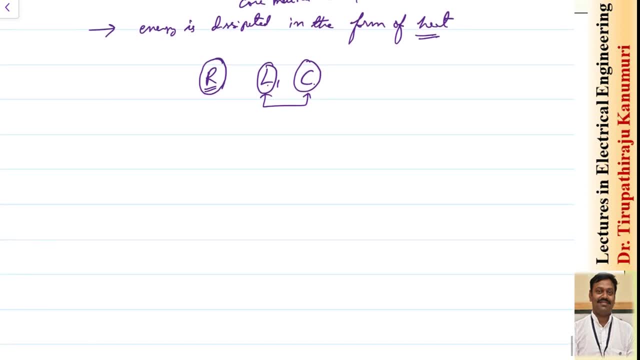 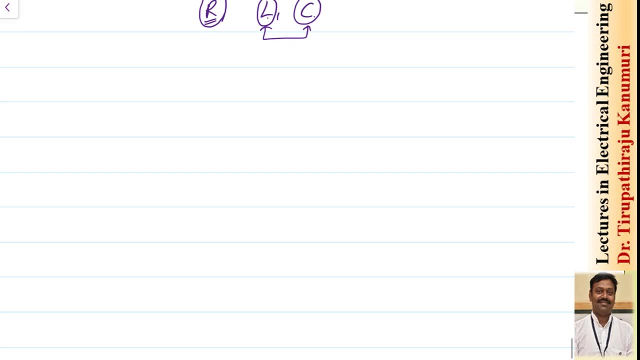 form of a resistance. They can be represented in the form of a resistance And these iron losses are independent of the load. That's why they are always represented as a shunt branch parameter. That means if you want to represent your transformer, so your transformer will be represented like. 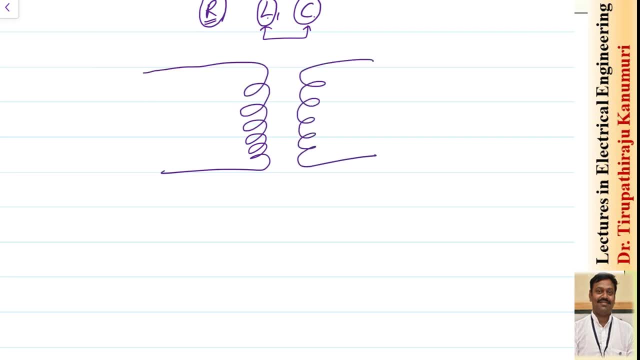 this. There is a primary and the secondary. Let's assume here the turns are n1 is to n2.. In some book you may see a parallel lines will be drawn between these core, but here when representing the equivalent circuit, because that core or iron component we are, 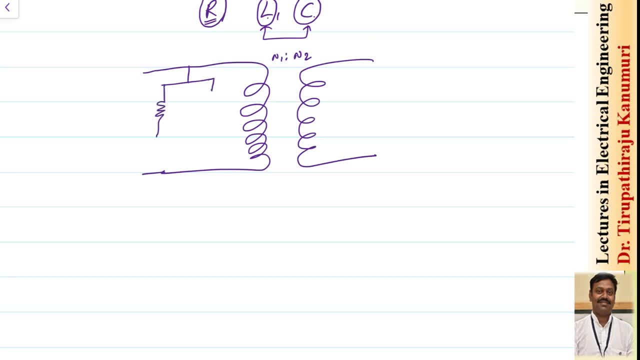 representing separately. so the first component is this iron loss component. so this iron loss component i can represent by a resistance known as r naught. it will draw a current that i am representing by iw or the watt full component of the current. so now this second component will be indicated by an inductor. this inductor reactance i am representing by x naught. 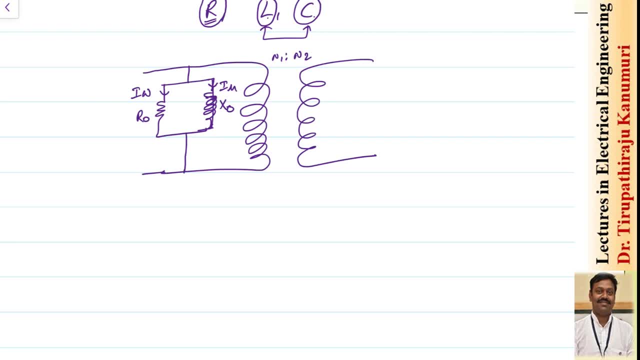 so this represent the magnetizing component of current taken from the supply. this is responsible for the production of flux, because last class i have proved that the flux is independent of the load and this iron losses. also they depends on the flux and flux intense depends on only voltage. so 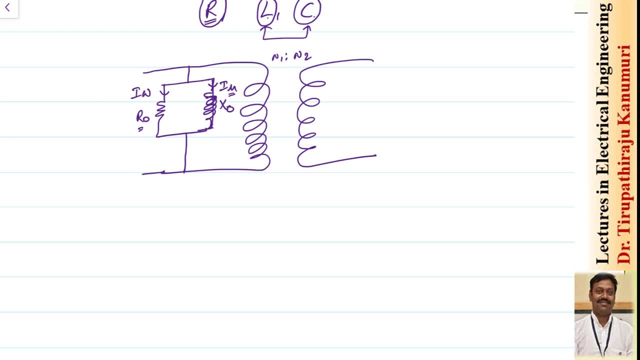 we can tell that this iron loss is also independent of the load. so the sum of these two currents gives my no load current i naught, so let us assume the primary voltage that is applied is equal to v1. so this way we have to represent here. you have to remember that this lines should not be there. 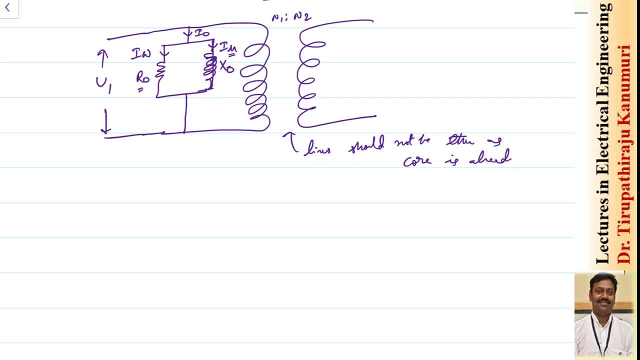 as core is already represented as shunt branch element. if the shunt branch element is not represented, then parallel lines will be drawn. here two parallel lines will be drawn like this. here these lines should not be drawn. please remember this, because some books make it general. these lines are drawn as shunt-branched lines only. scores before res, ordered in h's value from flux, that is the, and on x, a associated line, the last let's just writex by tc plus 1, and here the rise, which is percent, is into h. by ds power, and here plus here this is theійсьitch where order current was small: 했 to tg per part in cycle orích by h, 2 by m. the solar period values are: 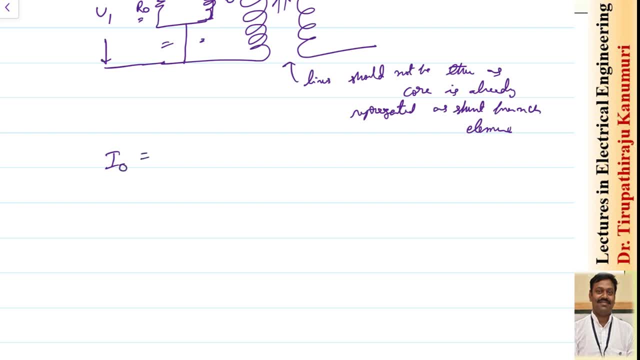 will Мнеzs the current vector and flavor, which is the test index into current growth and Kundralk condition, Tt. altrely we have a this mistake. So now this total current I can represent, I naught will be the phasor sum of: 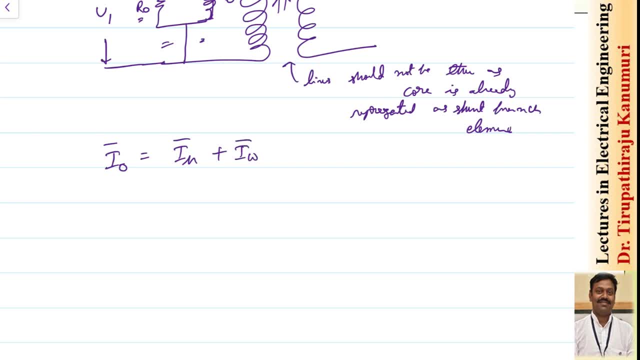 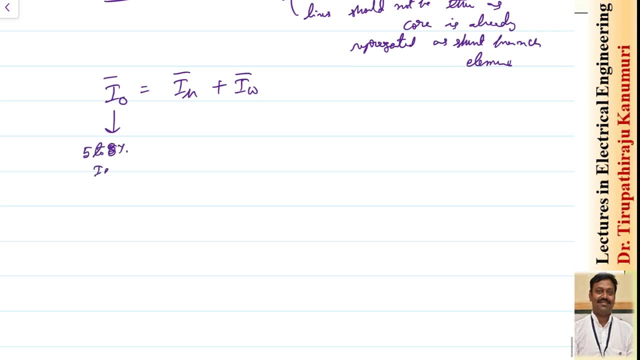 magnetizing component plus the waterfall component. So practically it is observed that the value of the no load current will encounter to 5 to 8 percentage of IFL and the magnetizing component will be 4 to 6 percentage of IFL and the waterfall component or iron loss component will be 1 to 2. 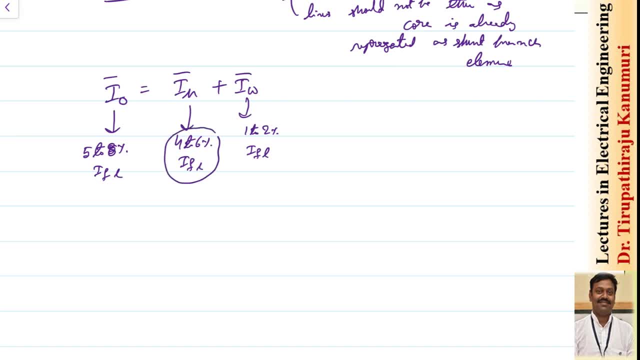 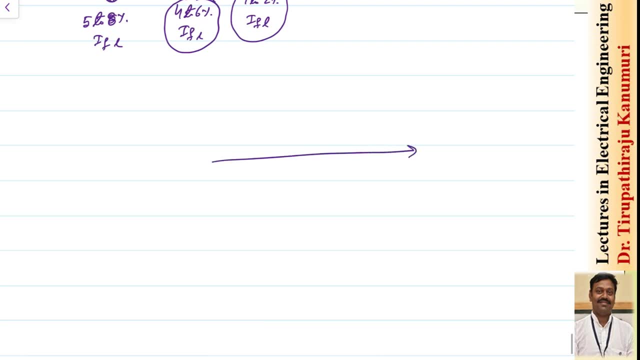 percentage of IFL, or we can tell the magnetizing component is more dominating when compared to iron loss component, So let us try to represent them. So if you are representing the flux here, So out of this the magnetizing component will be in phase with the flux or it is lagging your. 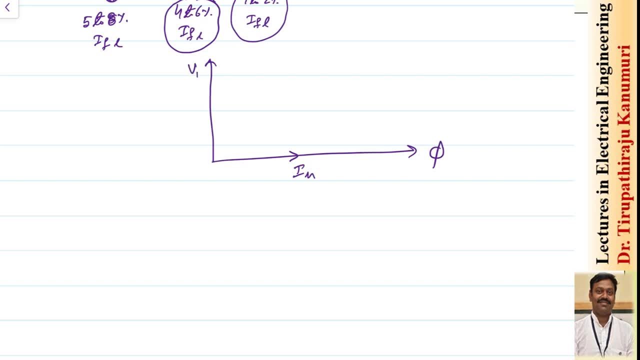 supply voltage by 90 degrees. So let us assume this is my voltage V1.. So this is my magnetizing component of current. So the waterfall component will be in phase with the voltage, because always the current passing through the voltage will be in phase with the voltage. So this is my magnetizing. 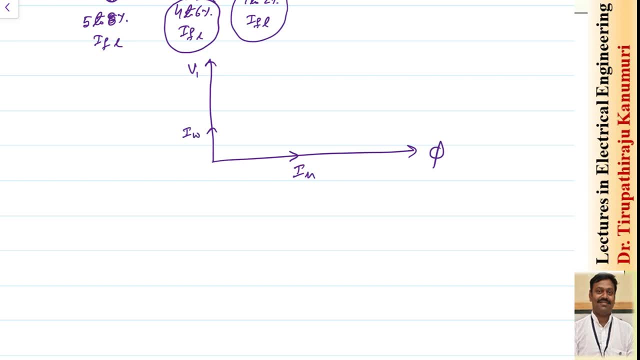 component of current. So the current passing through a resistor- this we have already seen in AC circuits. So same thing I am representing here. and in the inductor the current lags by 90 degrees. So same thing I have represented. So this resultant, or the sum of these two, gives the 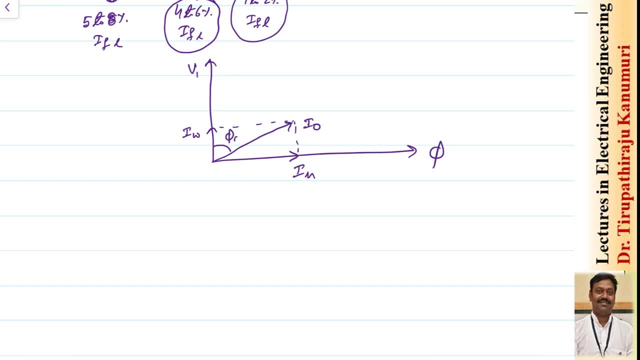 value of I naught or the no load component. Let us assume the angle with between voltage and this current I am representing by phi naught, So practically this value will vary from 70 to 75 degrees in practice, or we can tell that the cos phi naught, or which is the no load component. 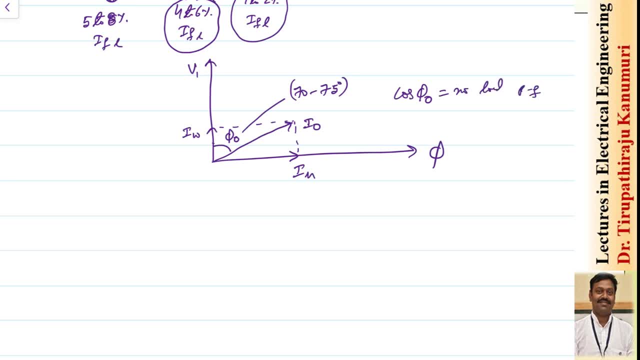 is also called as the no load power factor. This will be approximately equal to 0.2 and it will be lagging, So that is why it is represented by lag. So now the EMF induced are, as usual, this is E1. 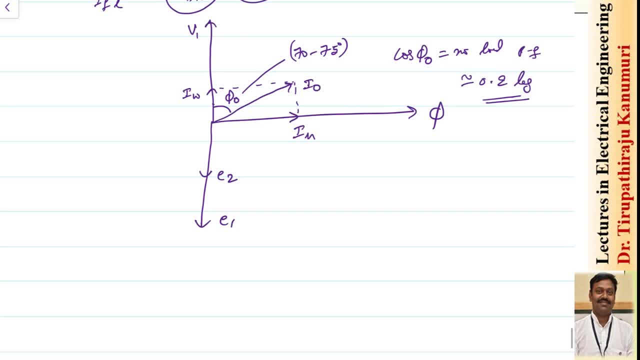 this is E2.. So this is the combined phasor diagram, which is combining both the finite permeability of the core, that is, IMU component, and the iron loss component, or IW component. I hope up to here it is clear to you. Now let us see when the semi-ideal transformer 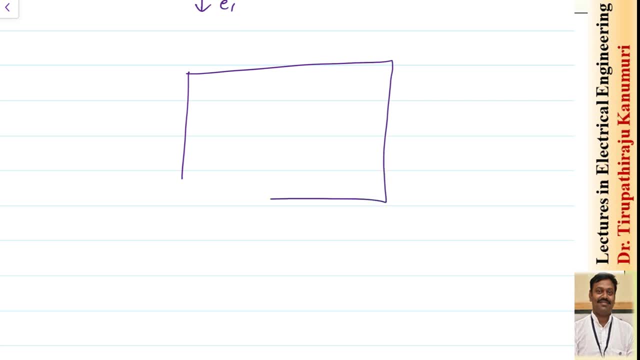 is connected to load, how it is going to behave. So I am taking the transformer again. So there is a primary winding and there is a secondary winding. So let us assume the secondary winding, the switch is open and there is some load that is connected and this primary is connected to some. 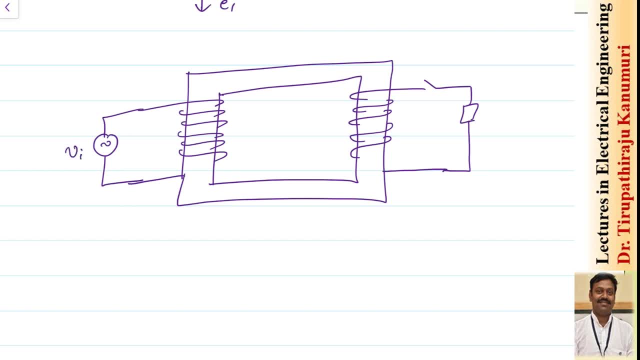 supply. So whenever the primary is connected to supply, let us assume the input voltage is there- it draws some magnetizing component. So let us assume that the input voltage is there. So if I draw the current I0, that means I draw the current I0.. Because of I0 the flux will. 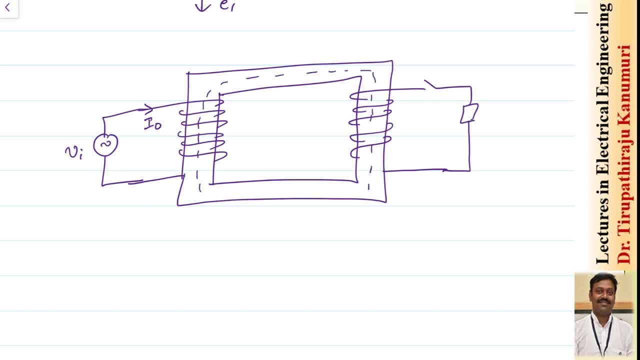 be produced in this core. So I0 is the sum of IMU plus IW. We have already discussed this one. Let us assume the flux that is passing in the core is 50 and let us assume the number of turns are N1 here. N2 is here because of this, EMF E1 is induced. here, EMF E2 is induced. 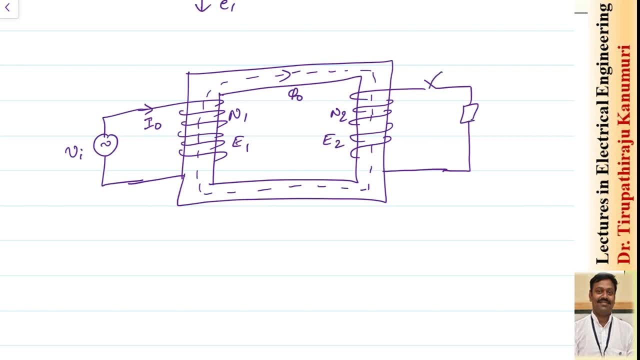 here that means EMF E2 is induced. So now let us assume the switch is closed. When the switch is closed, depending on what is the EMF e1 induced, here EMF e2 is induced, here is the impedance. the current will circulate in this loop because impedance, because e2 divided. 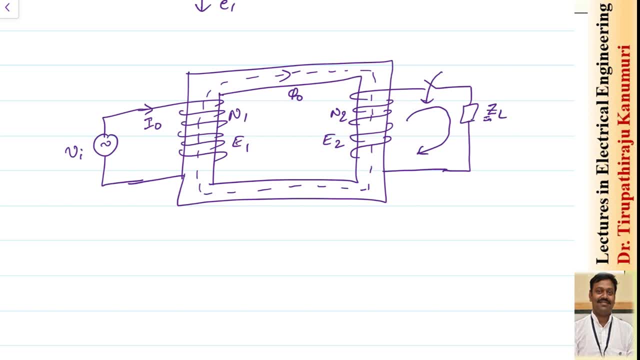 by the impedance. so let us assume zl is my load impedance. so this current i2 will be equal to e2 divided by zl. so based on that the current will pass. so now this current will lead to the magnetomotive force which is given by, because this current i2 is passing through n2 turns. so n2 i2. 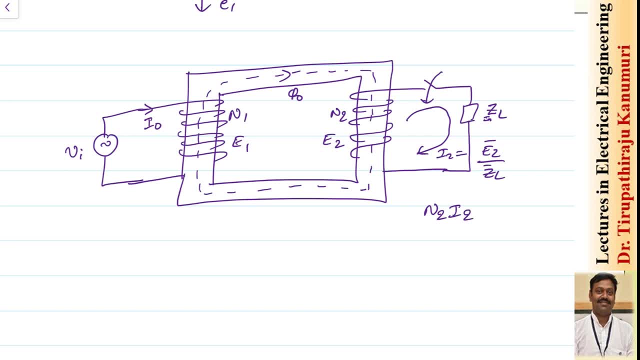 will produce one mmf and, as per the lenz's law, the current will pass. in such a way, it will oppose the cause. what is the reason for production of this? production of this one is phi naught. so it will produce a flux, phi 2, which will be opposite to phi naught. so whenever the flux phi 2 is there, 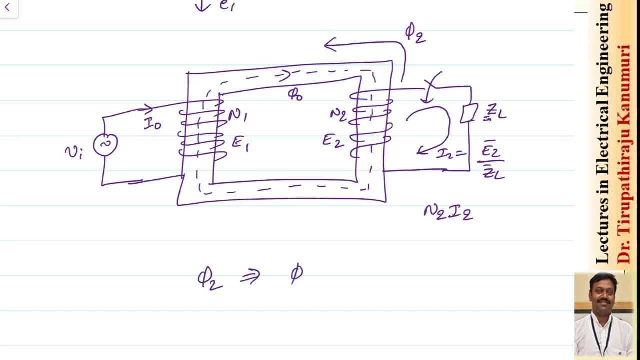 so automatically this leads to phi naught minus phi 2, so your net flux is decreased. when the net flux is decreased, obviously the value of e1 will decrease as well as the e2 will decrease. when the value of e1 is decreased to counterbalance or to satisfy the kvl, because e1 should come back. 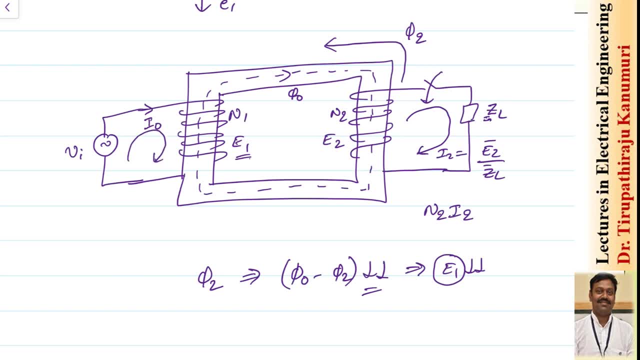 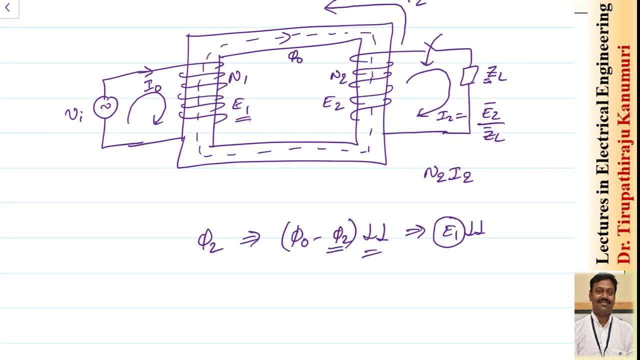 to its normal position, because if you apply the kvl in this loop, kvl should be satisfied. so what will happen? the primary will draw some extra current so that this phi 2 component will be cancelled out. so what it will do? it will draw one more extra component of current. i am 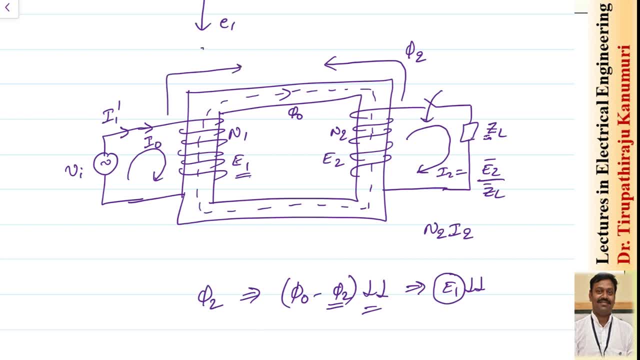 representing this by i1 dash. because of this i1 dash, a flux phi 1 is produced. that means n1 into i1 dash. one mmf of i1 dash is produced in this loop. because of this i1 dash, a flux phi 1 is produced. that means n1 into i1 dash, one mmf. 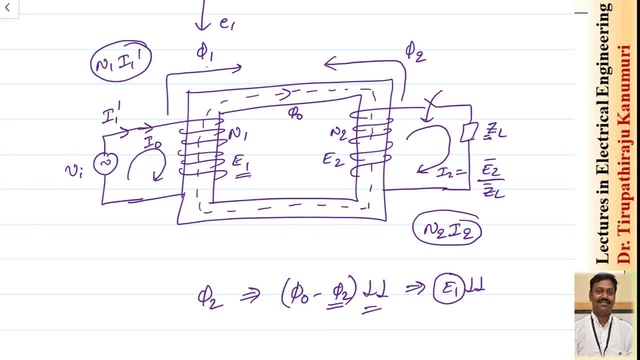 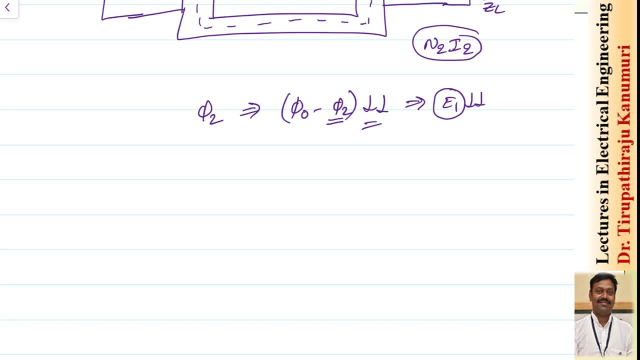 is produced by primary, which will counterbalance N2 into I2.. So primary MMF and secondary MMF will be counterbalanced. Getting it So because, as a result of this, so the net flux will be equal to phi naught minus phi 2 plus phi 1 dash, So these two are same, So this will become equal to phi. 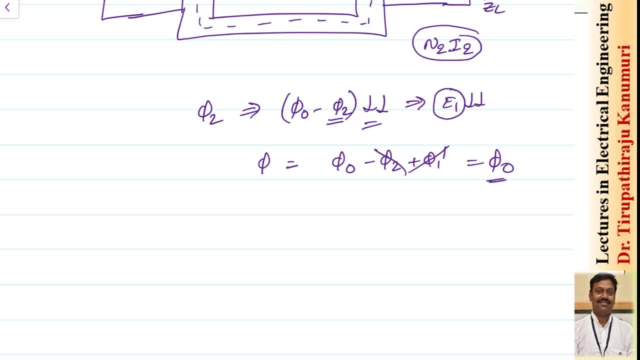 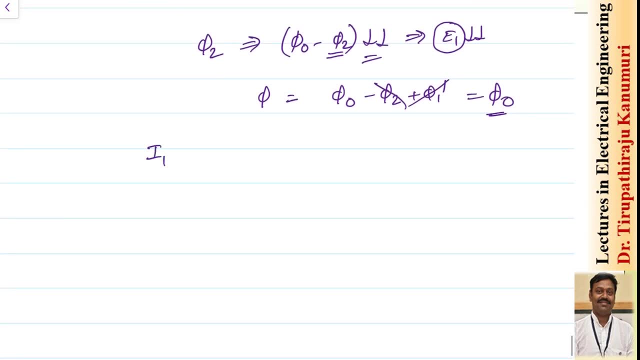 naught. So we can tell: the transformer is a constant flux device. The flux remains constant irrespective of load on the transformer. And now your total resultant value of the primary current will be the sum of the no load component of current plus the primary component of current. 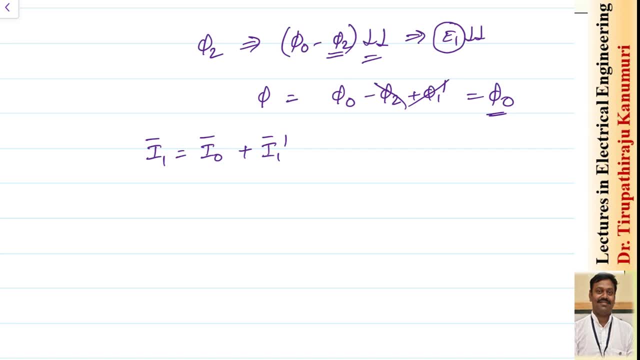 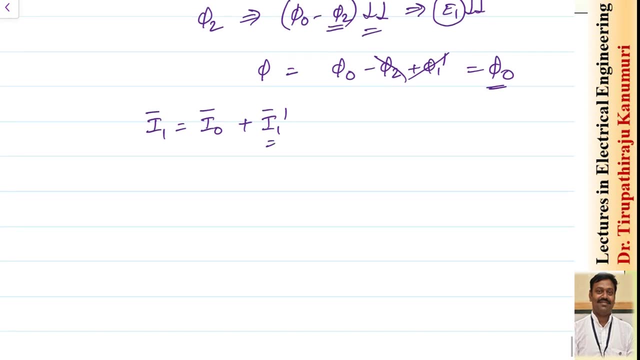 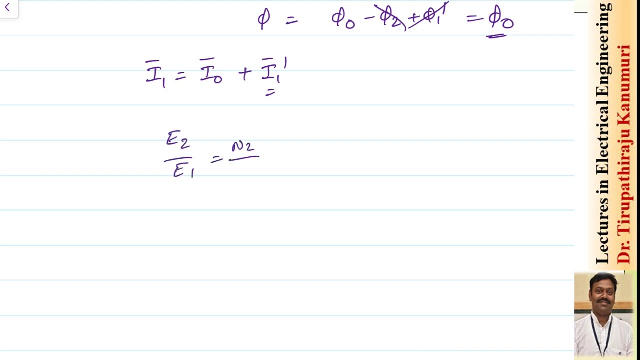 to compensate for the secondary component or the compensating component or the load component of the primary current. So that is represented by I1 dash. So from this relationship I can tell that E2 divided by E1 will be equal to N2. divided by N1 will be equal to I1 dash divided by I2.. This is equal to K. Previously. 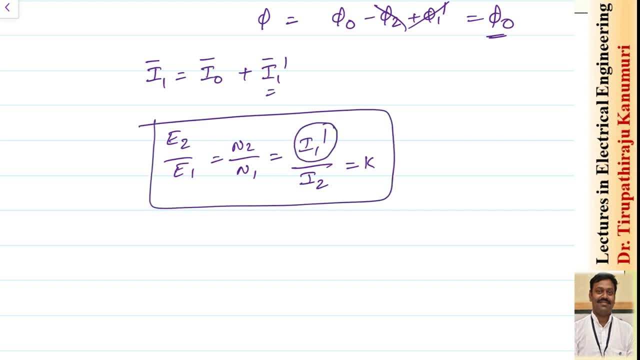 we have seen I1 divided by I2.. Here it is changed to I1 dash, not I1. So please remember this one. So now taking the phasor diagram of this one. So this will be like this: 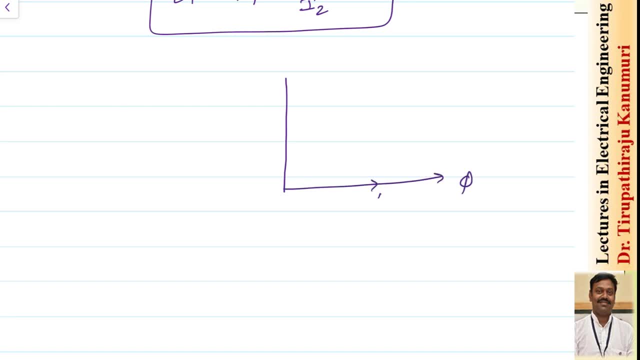 So this is my flux vector, flux phi. It is drawing a magnetizing component, I mu, and the watt full component I w. Because of this there is a no load component of the current, Because here I am representing in the bigger size. practically the value of I0 is only 5% of. 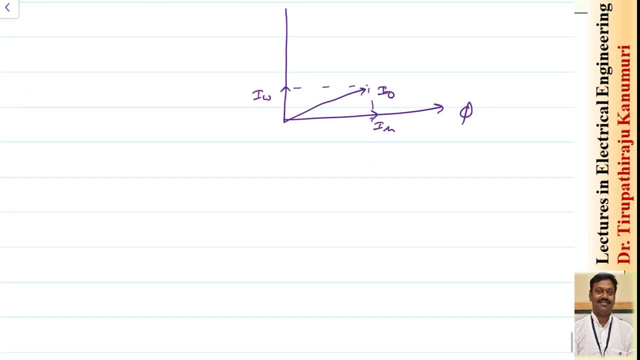 the value of the I1 dash. Please remember this one. So because of this I mu or the flux, the EMF is induced in the secondary side, that E2 will be equal to V2.. Let us assume when the load is connected, that load is a lagging power factor load. It can be leading power factor or unity.